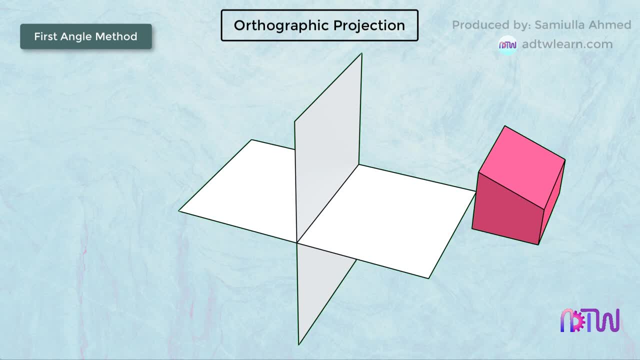 First angle method. In the first angle method, the object is placed in the first quadrant such that it lies between the viewer and the plane of projection. While considering the observer is standing here, view from this point is considered as the front view. When the viewer views the object from the front view, its projection is projected on the 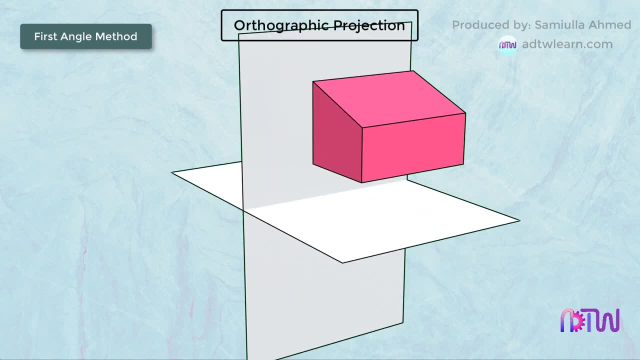 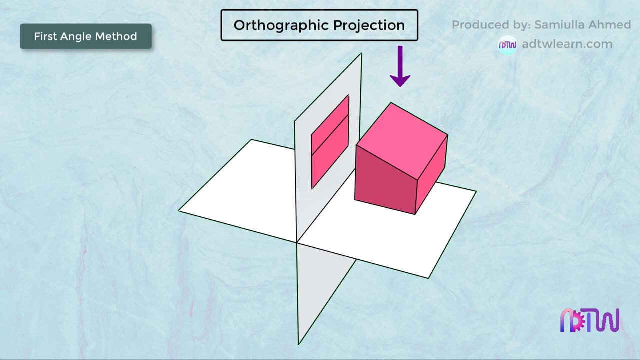 vertical plane of the first quadrant, You can see from the viewer's eye how the front view of this object looks. And when the viewer views the object from the top, its top view is projected on the horizontal plane of the first quadrant. This is how the top view looks from the top For the left. 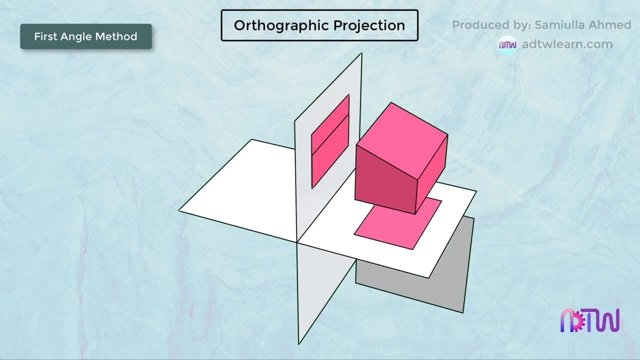 hand side view. we consider another parallel plane which is placed on the right side of the object And when the viewer views the object from the left hand side of the object, the left hand side view is projected onto the profile plane. This is how it looks For the right hand side view. 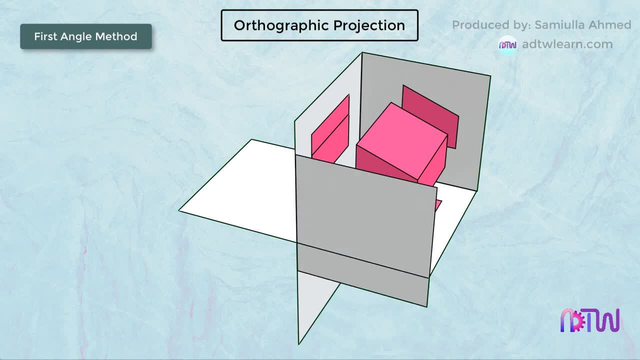 we consider another parallel plane on the left side of the object And when the viewer views the object from the right hand side, its top view is projected on the left side of the object. The right hand side view is projected onto the profile plane which is placed on the left side of. 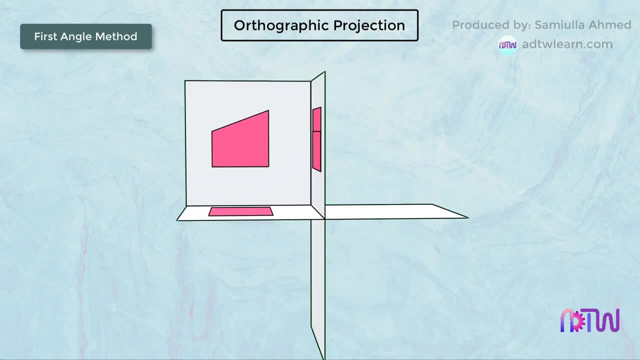 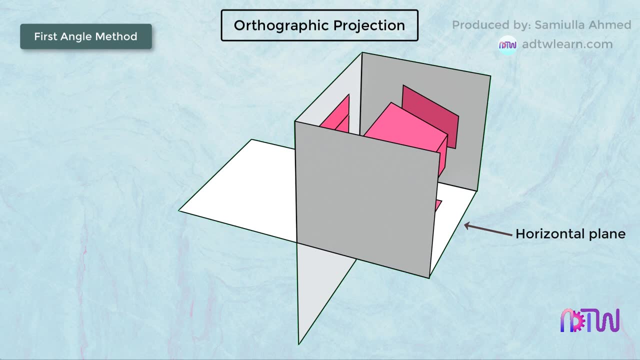 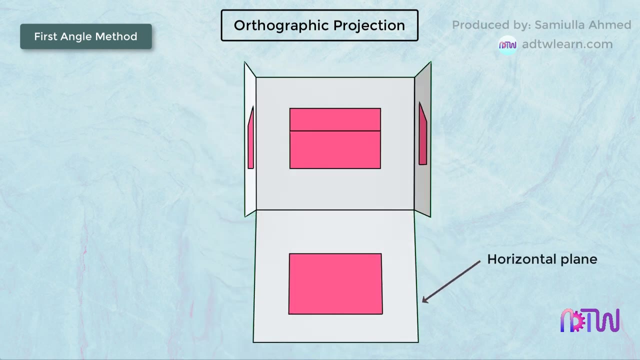 the object. This is how it looks. For drawing these projections onto the drawing sheets, we follow the rule of orthographic projection. According to this rule, to draw the projection of a 3D object on the 2D plane, the horizontal plane is rotated in the clockwise direction and 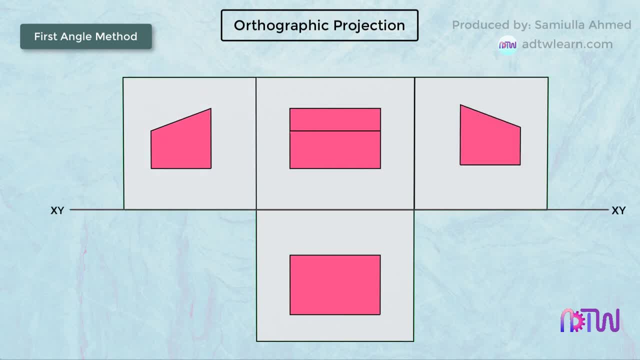 the profile planes are also unfolded. By doing so, we have the following projections: The front view of the object is on top, the top view is on the bottom, the left hand side view is on the right side of the front view and the right hand side view is on the left side of the front view. 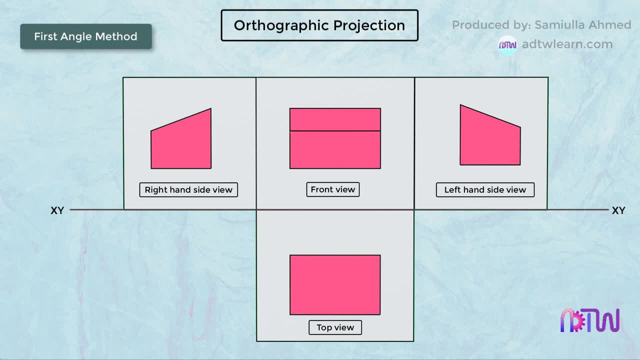 This is how we draw on drawing sheets, using the first angle method. If you are enjoying this video, please give this video a thumbs up, as it helps the YouTube algorithm to recognize good content and suggest others who want to learn. and if you are new to ADTW, Learn, click on the. 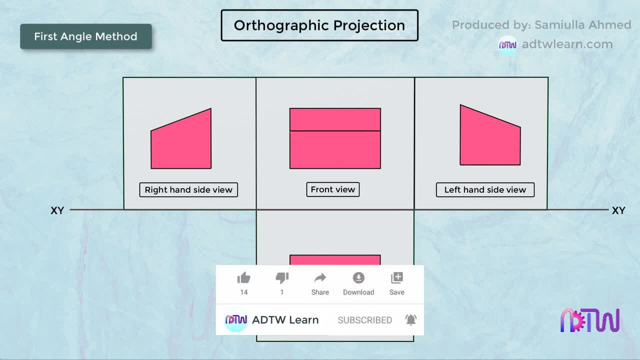 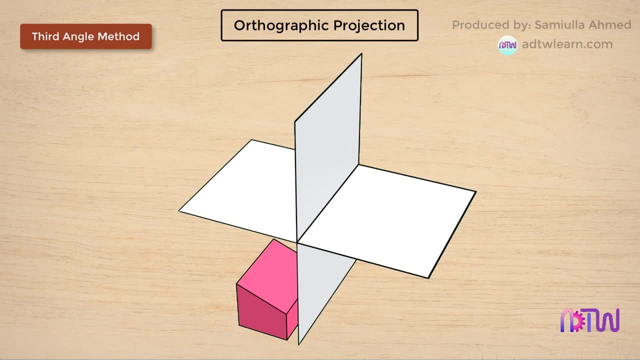 subscribe button and turn on the notification to get more informative videos like this Third angle projection method. In this projection method, the object is placed in the third quadrant and the plane of projection lies between the object and the viewer As the vertical plane. 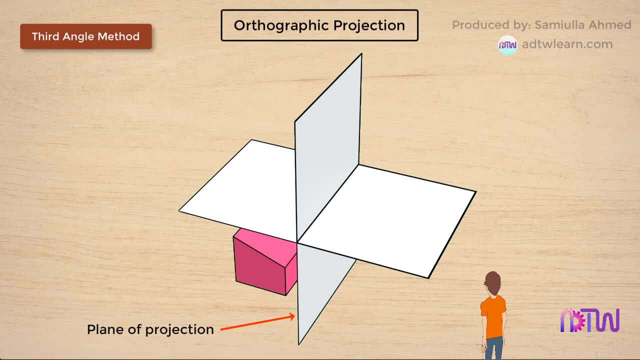 of the third quadrant lies between the viewer and the object. the viewer cannot see the object. Therefore, we will make the vertical plane transparent and then we can see the front view, which will be projected on the vertical plane lying between the viewer and the object. 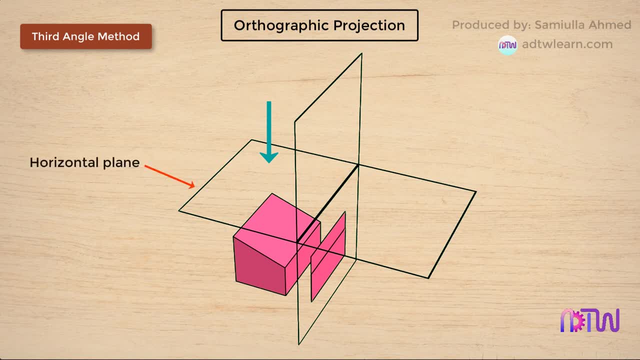 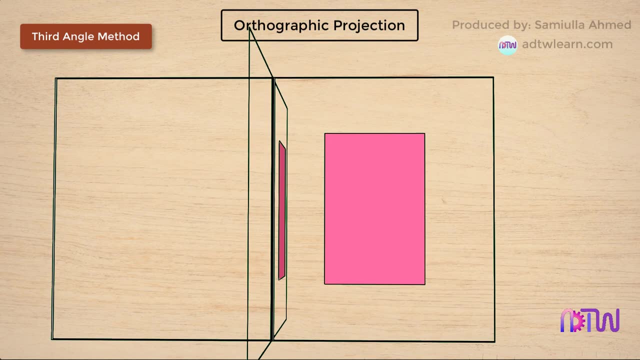 Similarly, while viewing from the front view, the horizontal plane will come between the point of view and the object. Therefore, the top view will be projected on the horizontal plane. For the right-hand side and left-hand side view, we will have the two profile planes on. 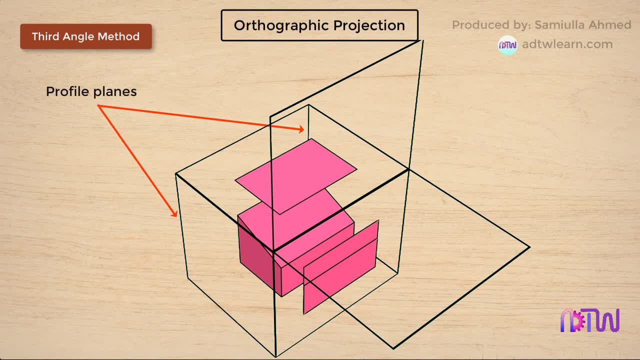 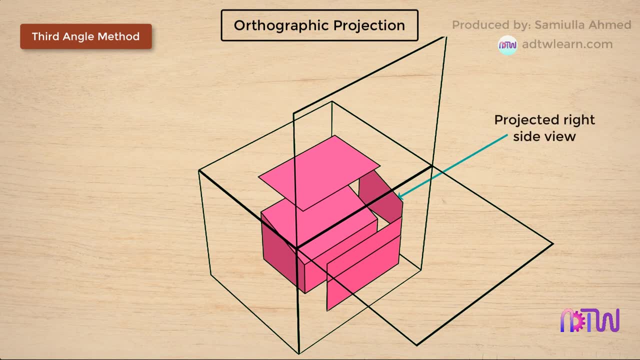 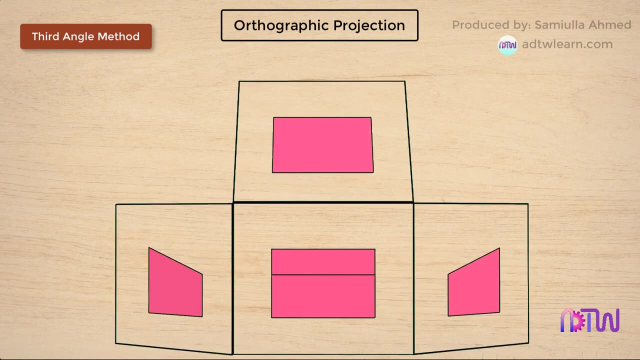 either side of the object. Now, when the viewer sees from the right side, the right side view will be projected on the right profile plane of the third quadrant and the left side view will be projected on the left profile plane. block Government. When we unfold the planes according to the orthographic rule, 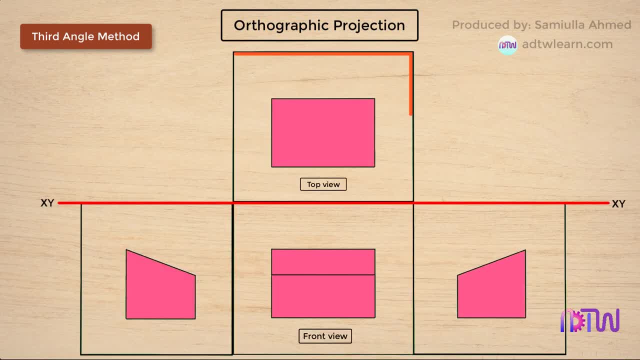 we will get a front view on the bottom of the xy line, a top view on the above xy line and left side view on the left side of the front view and a right side view in the right side of the front view. This is how first and third angle projection method works. 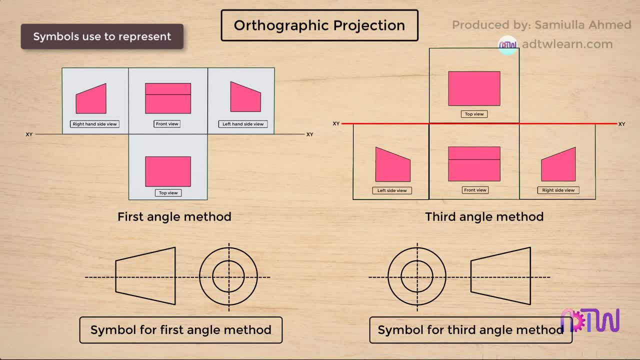 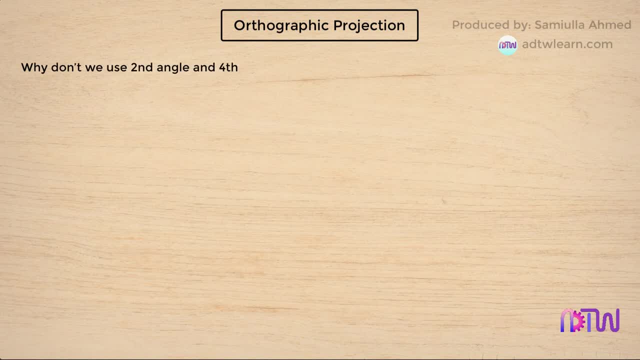 Symbols used to represent. These are the symbols used for representing first angle and third angle method: rectangular: cuánt hau, mustardes, sault. Automatic parameter. second angle and fourth angle method. it is not possible to show a 3D view of an object on the 2D. 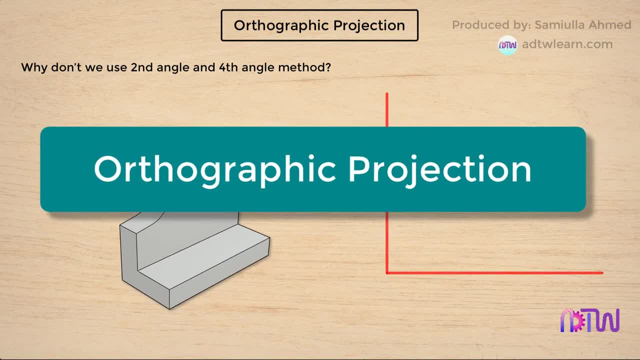 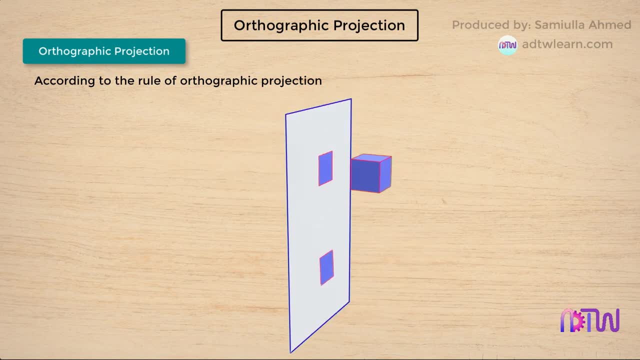 plane. therefore, we use orthographic projection. According to the rule of orthographic projection, the horizontal plane needs to be rotated in the clockwise direction to view the top and front view on the 2D plane. Once the horizontal plane is rotated in the clockwise direction, 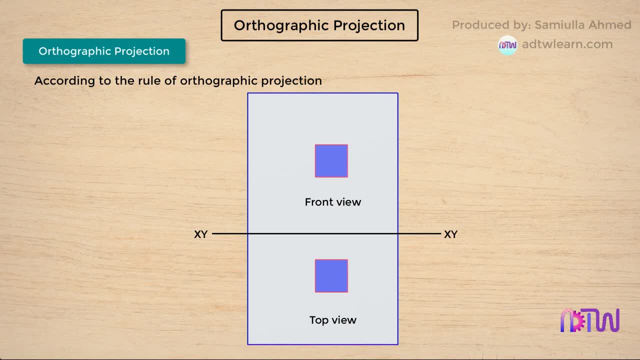 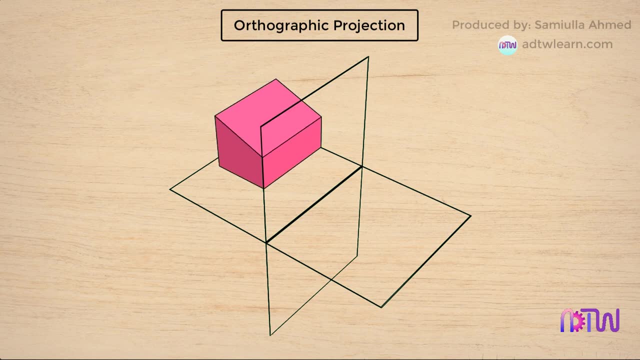 the projections present on the horizontal plane are also rotated along with the plane. Now consider the second angle view, in which the object is placed on the second quadrant and the plane lies between the object and the viewer. The top view is projected on the horizontal. 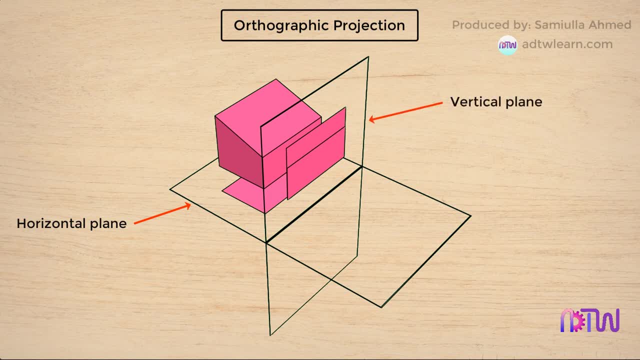 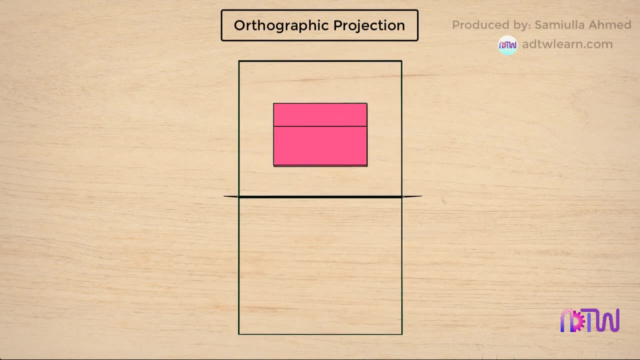 plane and the front view is projected on the vertical plane, and when the horizontal plane is rotated in the clockwise direction, the top view projected on the horizontal plane will overlap with the front view projected on the vertical plane. A similar problem will occur while using 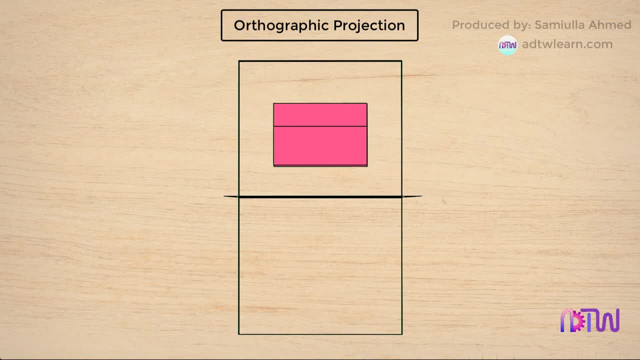 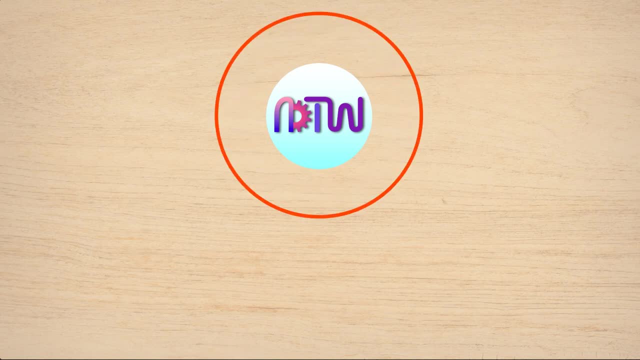 the fourth quadrant. Therefore, we don't use the second and the fourth angle method. I hope you have understood the first and third angle methods. It takes lots of effort to make such informative videos. You can help ADTW learn to make more videos by joining our channel and. 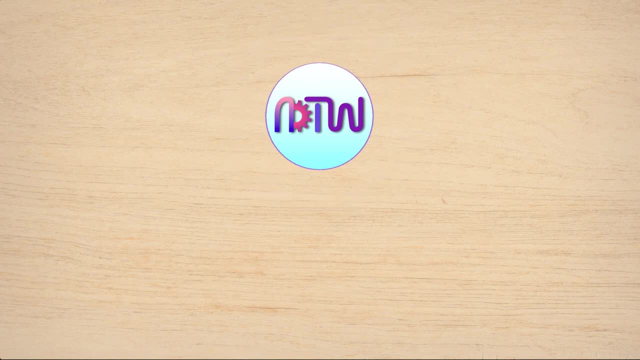 contributing to developing more such videos. Your support will help us make great educational videos. Other ways of helping us is by sharing our videos with your friends. Thank you. 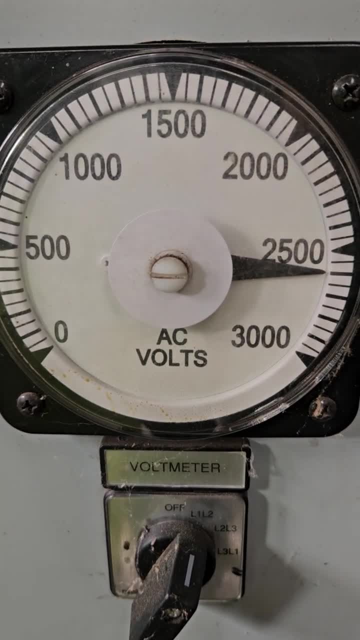 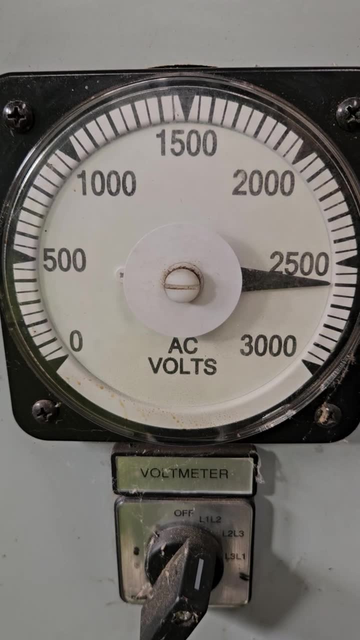 James asked about how we measure high voltage from the generator. He guessed that the meter isn't hooked up directly to the output and that there's some special circuit stepping down the power so that it's readable. He wanted to know if he was correct. Here you go, James. This is 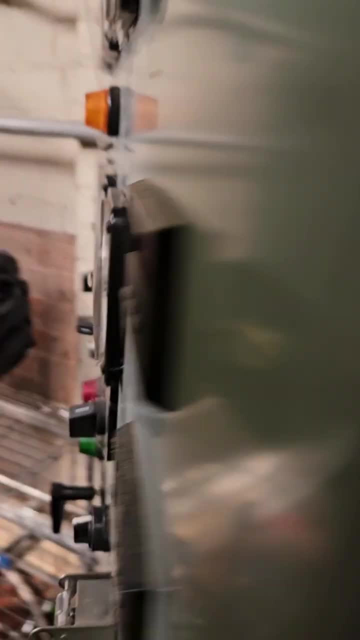 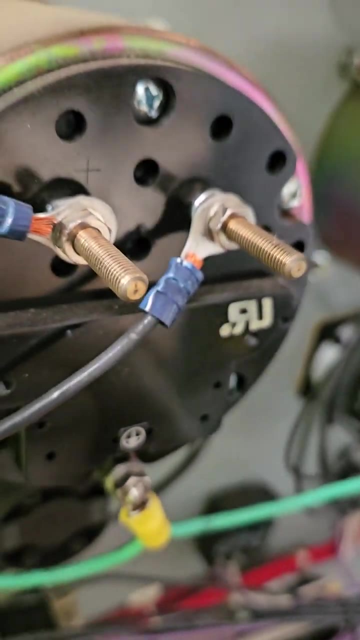 one of our volt meters. The scale is up to 3000, but let's have a look at the back of the meter. See those terminals. No big bushings means these are low voltage connections. This meter isn't actually designed to read up to 3kV. In fact, if you hooked it up to that kind of voltage, 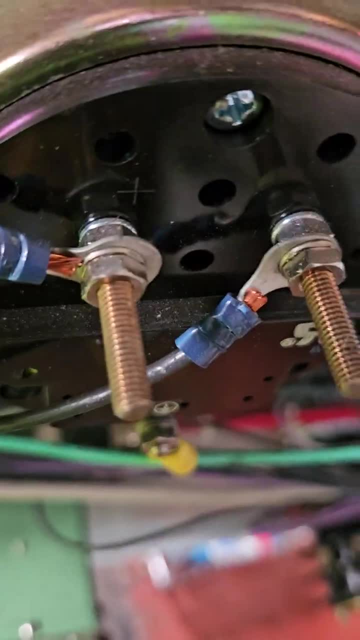 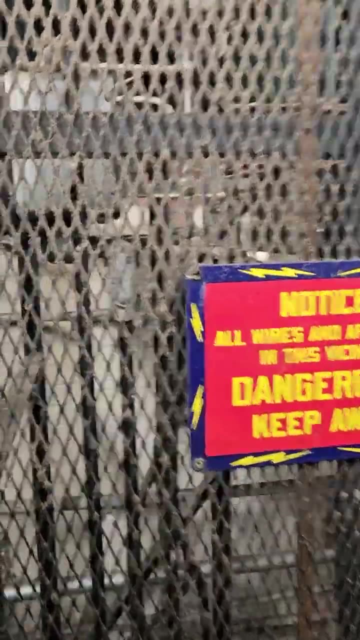 it would absolutely release the factory-installed magic smoke that makes it operate. It's intended to be used with what we call a PT, a potential transformer. That's a special type of transformer designed to drop the voltage from high bus voltage down to something safer to work with Most meters. 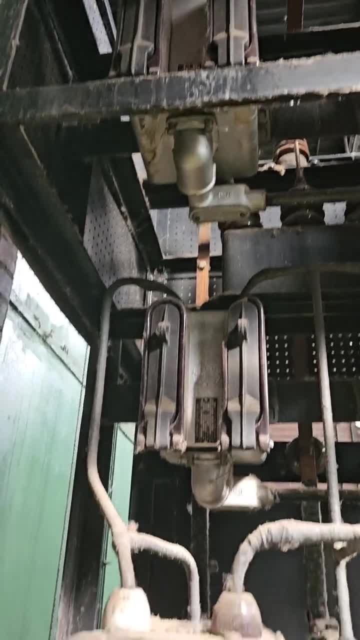 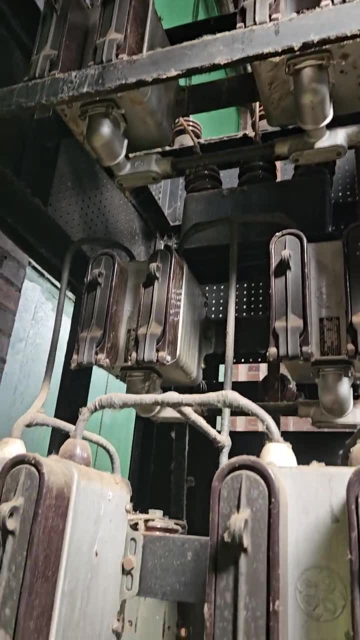 work in the 120V range and potential transformers come in a variety of fruit flavors to fit them. We'll dig deeper in a long-form video on this channel. but to answer your question, here's some antique examples- the oldest in my fleet I came here today to give you a look at. 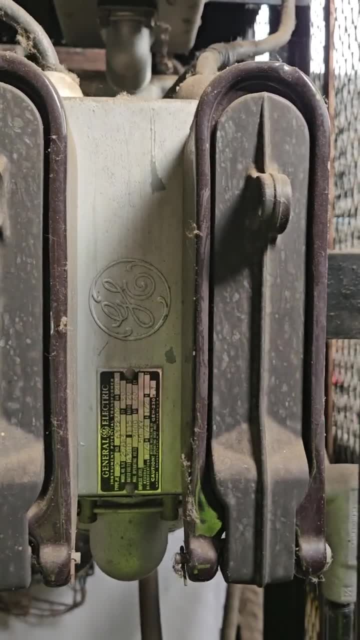 them. This is a whole array monitoring all three phases of our main bus. Examine the setup here and try to work out what's going on. I'm sure some of the old guard will have a field day answering this. I'm sure some of the old guard will have a field day answering this. I'm sure some of the 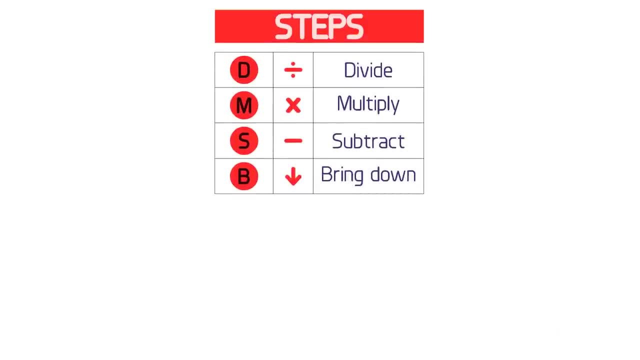 Long division is a step-by-step method for dividing the multi-digit numbers. It involves four basic steps: Divide, multiply, subtract and bring down- and then, repeating the process, Use the acronym DMSB, which stands for divide, multiply, subtract and bring down It.